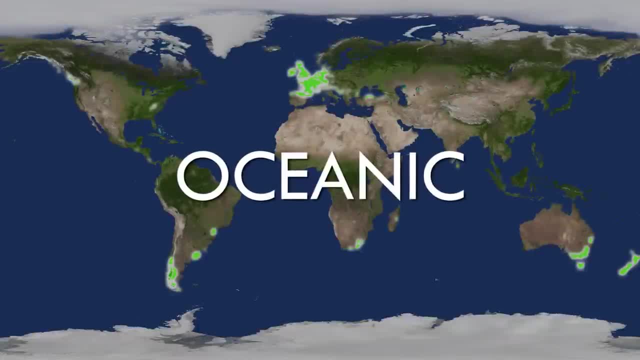 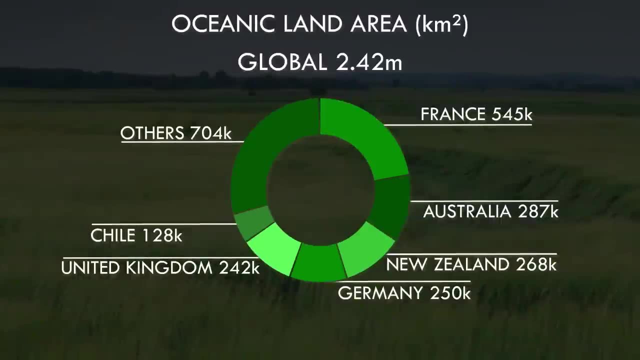 At number 11, we have the next largest zone, that of the oceanic, The mild, wet climate found on the west coasts of the continents at temperate latitudes. Most of the land area is found in northwest Europe, with a significant proportion in Oceania. The main variant of 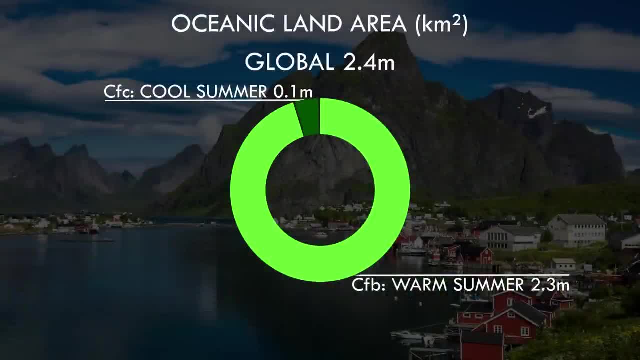 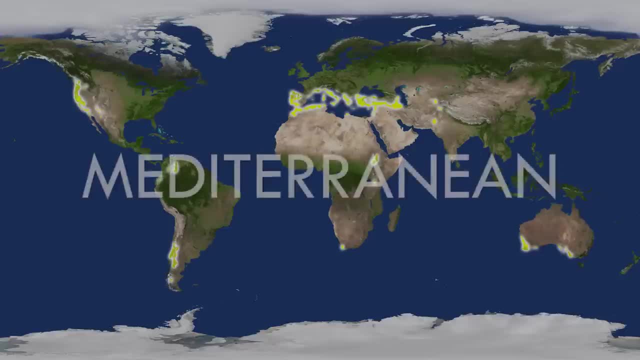 warm summers dominates, with the cool summer subpolar variant restricted to rocky coasts in the far north and south. At number 10, we have the oceanic southern neighbour, The Mediterranean climate of dry summers along the west coasts of the temperate latitudes. 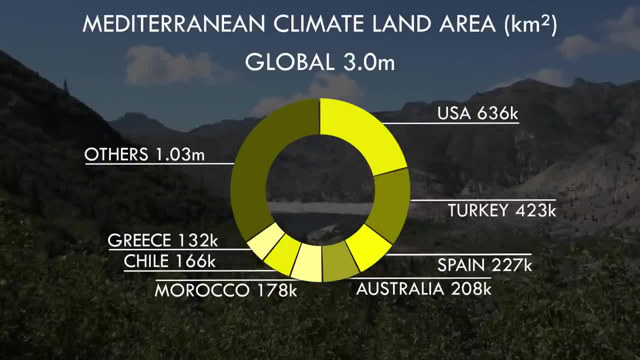 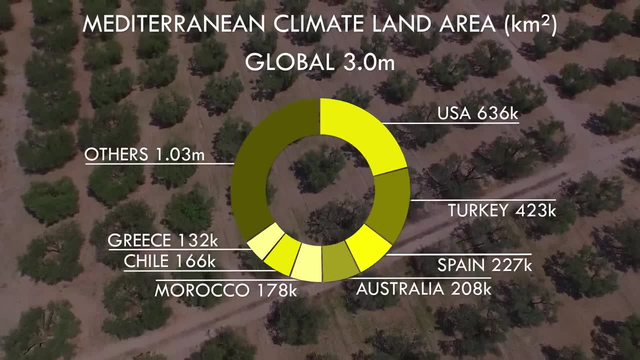 The country with the largest single land area here is, interestingly, the United States, whose long west coast is almost exclusively of this type. Australia and Chile have some areas here, but the vast majority is given over to the countries around the sea to which 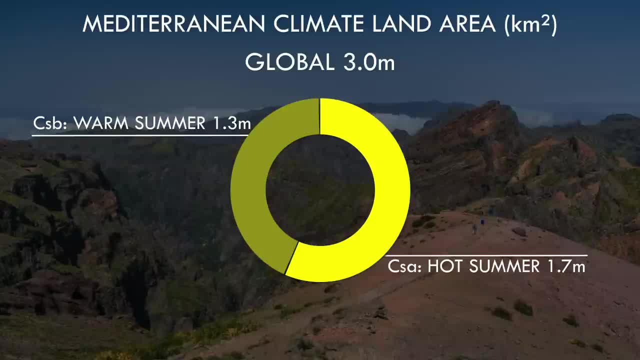 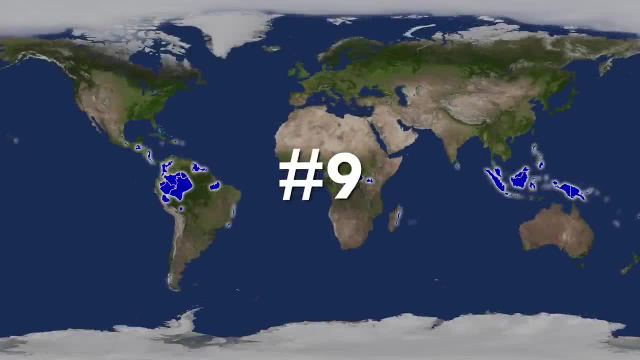 this climate owes its name. The relative land areas of the hot and warm variants of this climate are pretty even, with CSA being slightly more widespread. The next largest climate type, at number 9, is the tropical rainforest, covering selected parts of the equatorial regions of our planet where rain is constant year round Almost. 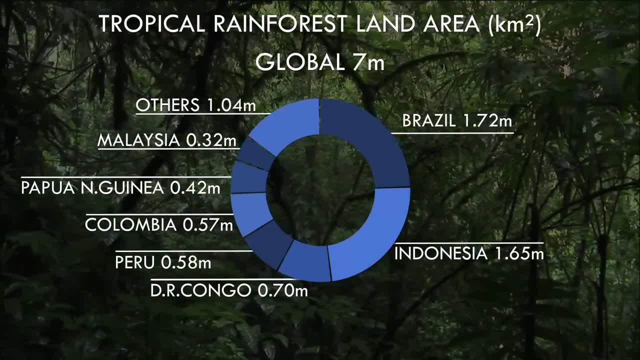 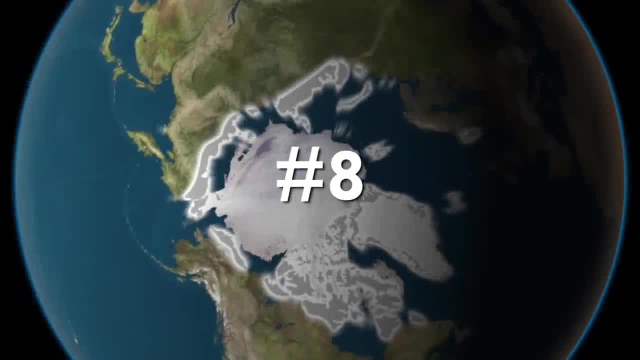 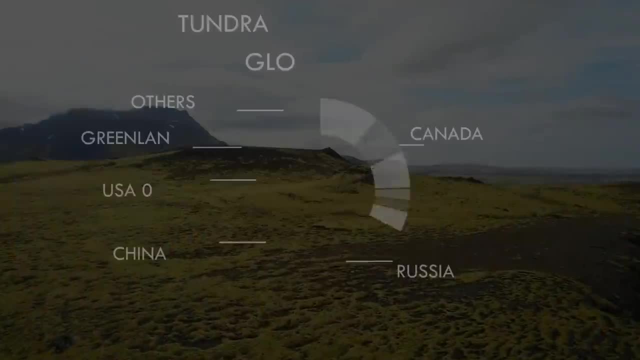 half of this area is within Brazil and Indonesia, with the remaining countries scattered across South America, Africa and South East Asia. Moving onto number 8 now and we switch to the opposite end of the earth and the opposite in terms of temperatures. with the frigid wastes of the tundra, Most of this land is. in the arctic, with over half of it in just two countries, with the arctic being the largest of the arctic. Most of the arctic is in the south, with the arctic being the largest of it. The arctic area is in the north and the arctic area is in the south, with the arctic 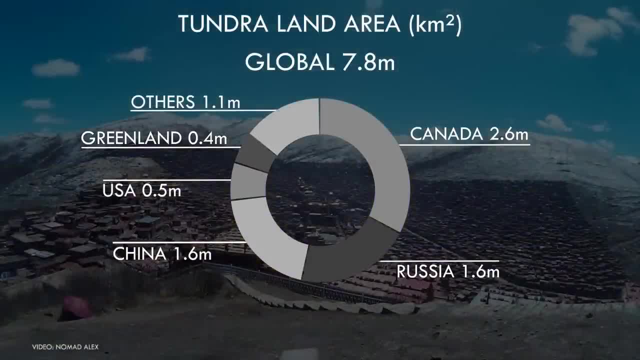 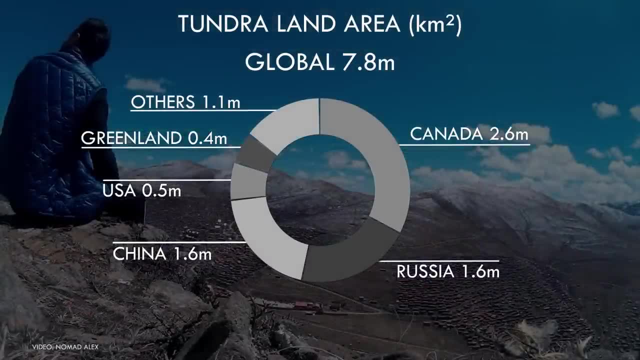 Russia and Canada. You might be wondering what China's contribution is all about here. Well, that's the extensive Tibetan Plateau which, being at an altitude of over 20,000 feet, is predominantly alpine tundra. The United States fraction here is almost all from one state. 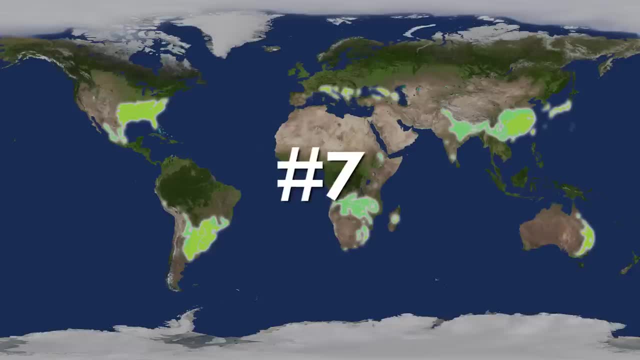 Alaska On to number seven in our climate land areas list and we have the climate zone that has the largest population of any other: the humid subtropical of hot summers and cool winters mixed with plenty of rain, occurring on the eastern fringes of each continent. Almost half of the 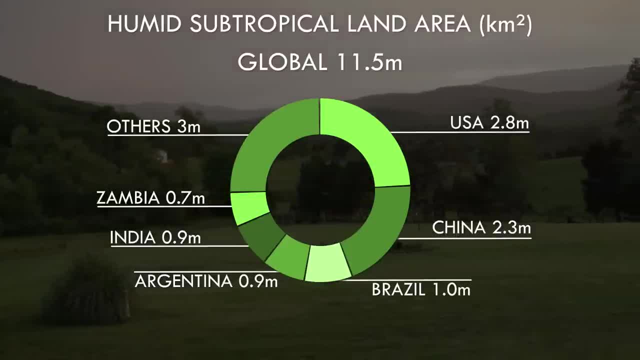 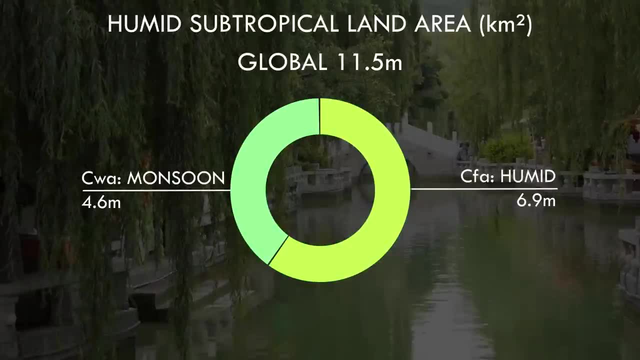 global land area of this type occurs in just two countries, the United States and China, with the rest scattered across other continents. The year-round rain variant is the larger of the two, with the smaller being the monsoon form, with dry winters Into the final six now, and we have 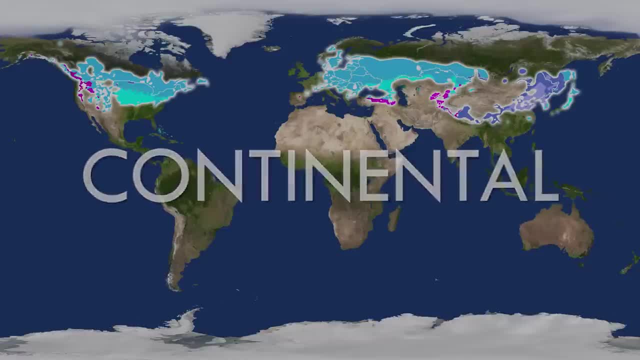 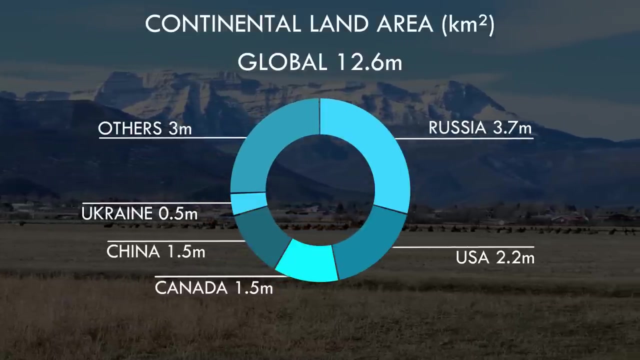 the continental climate types which stretch across the vast plains of North America and Eurasia at the mid-latitudes, characterised by warm to hot summers and cold winters, but with adequate rain to support large populations. This climate type forms the heartlands of three countries: Russia, the United States and Canada, which together make up over. 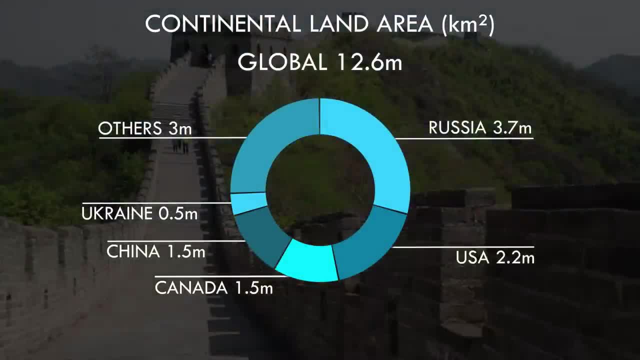 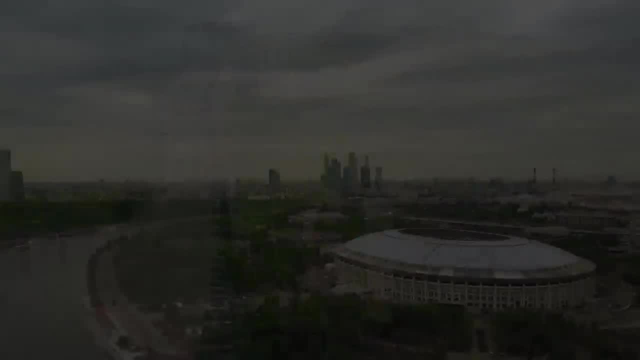 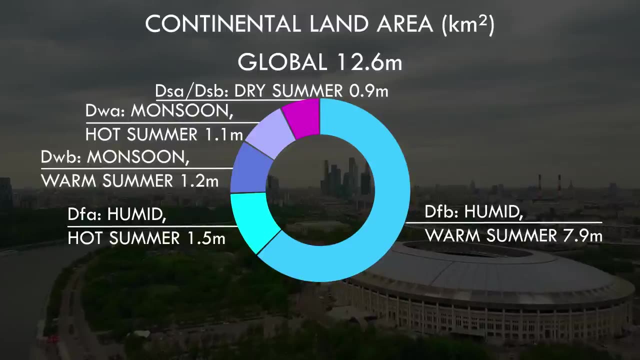 half of all global area. for this climate type, China's densely populated northeastern part features also, with the remainder being in Eastern Europe and Northeast Asia. There are many subtypes to this climate, varying by summer temperatures and annual rainfall distribution. A single type dominates, however: that with year-round precipitation. 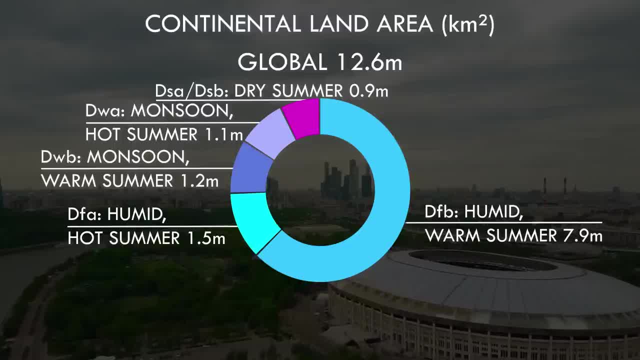 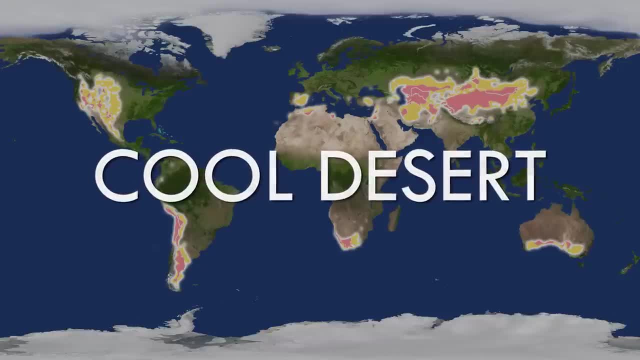 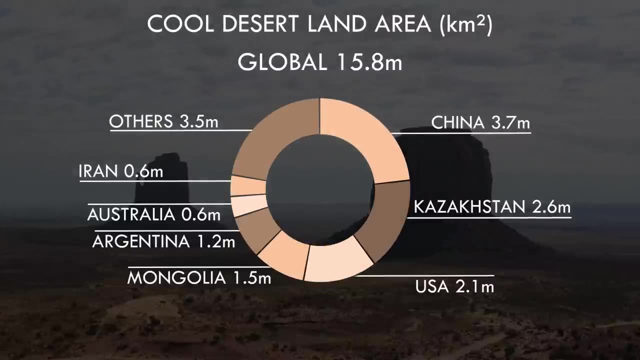 rain in summer, snow in winter, together with a warm summer. The fifth largest climate zone is the cool desert stretching across the rain-starved continental interiors, where large temperature ranges in combination make for a tough existence. Most of this area is covered by the countries of Central Asia, with most of western China in 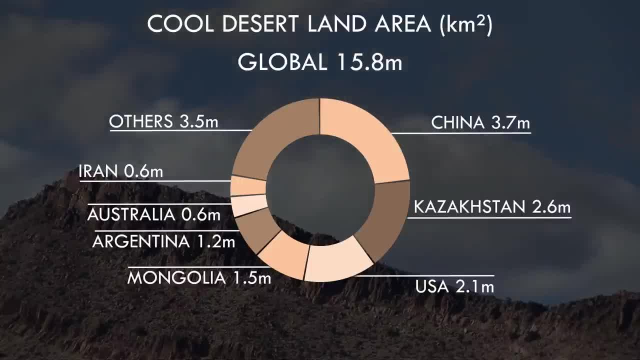 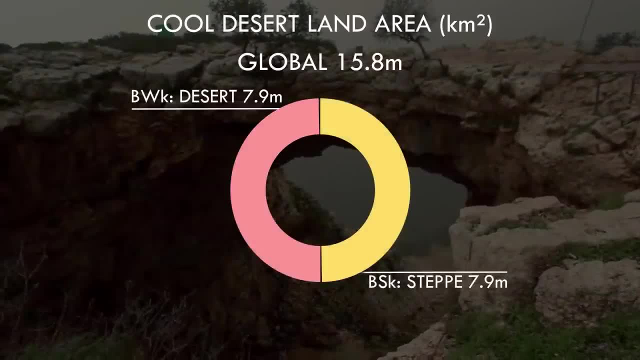 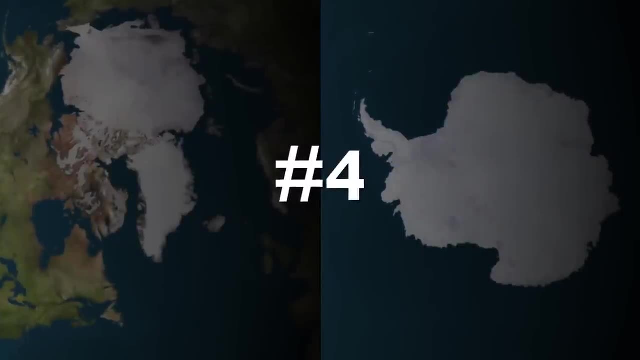 this category. Similarly, most of the western half of the United States is comprised of this climate zone. The remainder are scattered across the other continents. The true desert and semi-arid forms of this climate are equally matched in prevalence Onto number 4, and no, it's not been forgotten, It's the most forbidding of all climate zones. 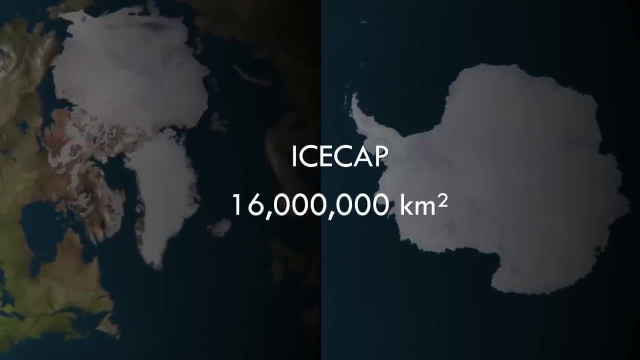 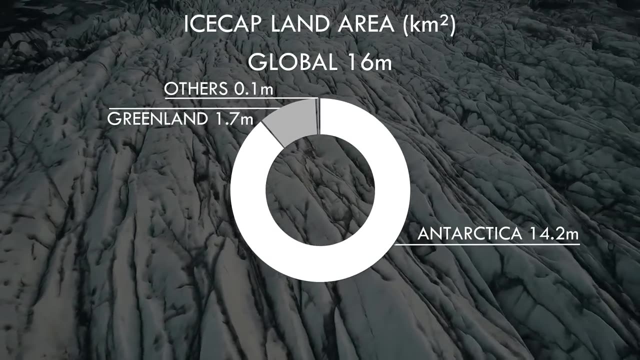 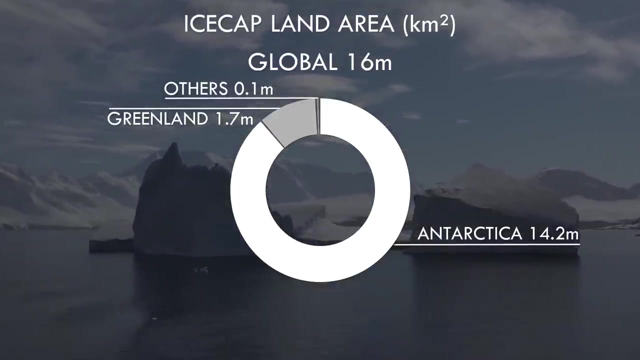 the ice cap. Almost the entirety of the large continent of Antarctica is covered in ice year round, And this continent alone makes up the vast majority of land area of this climate type, with the remainder being in Greenland and a comparatively tiny scrap as glaciers across the highest mountains in the rest of Earth. 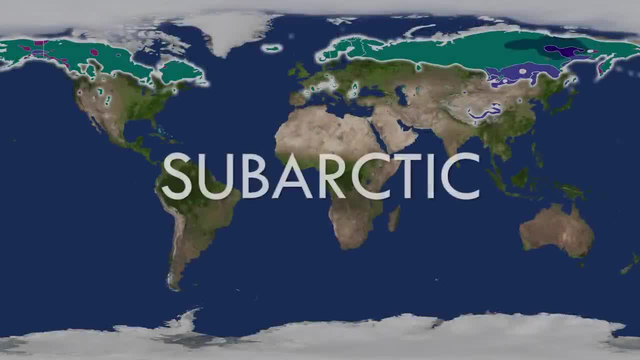 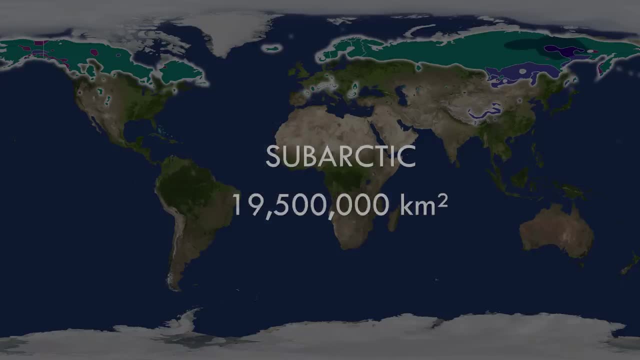 As we move to number 10.. Number three, and we have the climate zone with the next coldest winters – the vast boreal forests of the subarctic that cover 12% of the entire land area of Earth, Dominating the northern continental interiors of North America and Eurasia. it is no surprise. 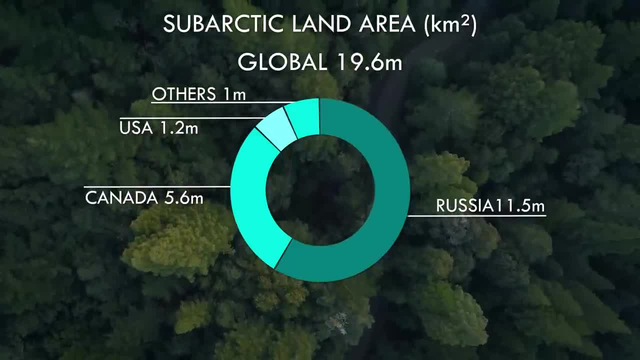 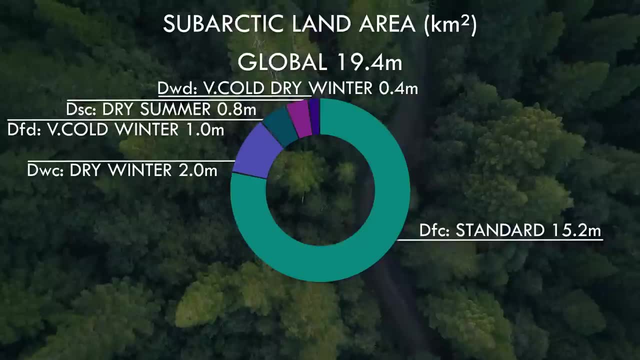 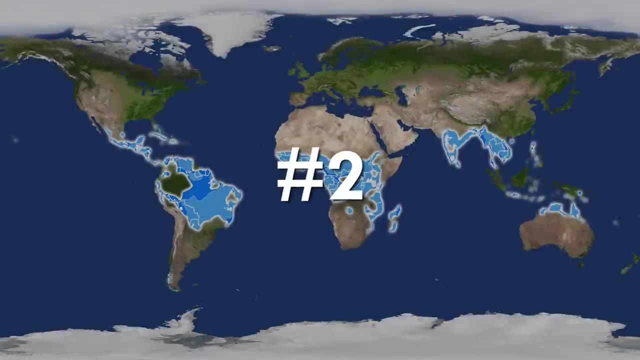 that just two countries make up the vast majority of this land area – Russia and Canada. The variant with cold winters and year round precipitation dominates this climate type, with monsoon and very cold winter forms comparatively isolated Onto number two in our climate land areas list and we are back in the tropics with 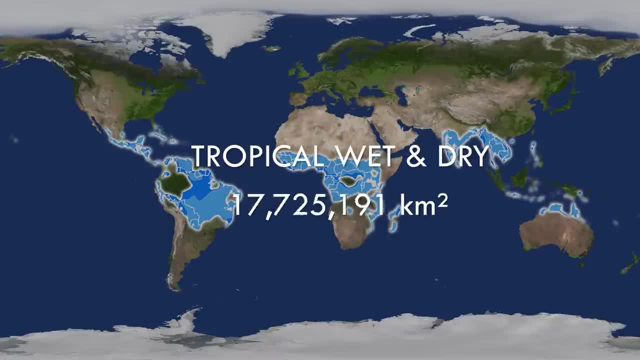 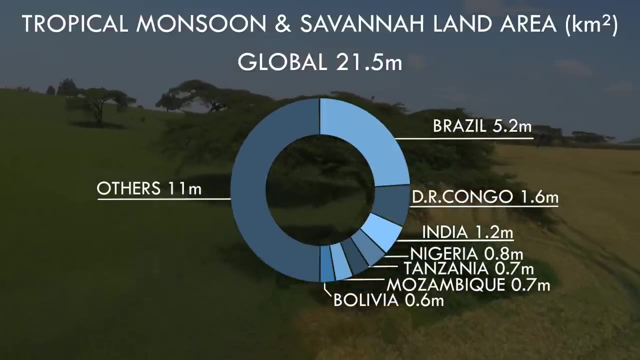 the wet and dry seasonal climates – the tropical monsoon and tropical savannah. These lands dominate the tropics, making up almost 75% of land area in this region of Earth, with the tropical rainforest making up most of the remainder, Although the vast savannah of Brazil makes up almost a quarter of this climate's land. 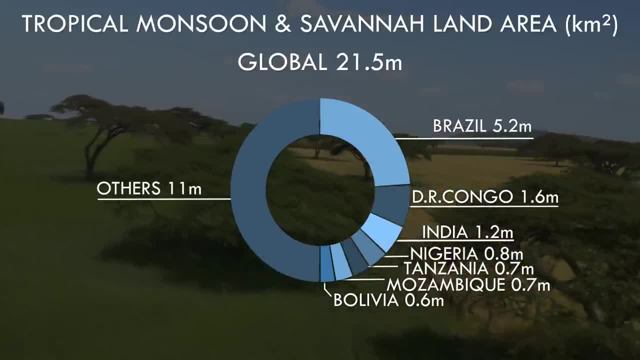 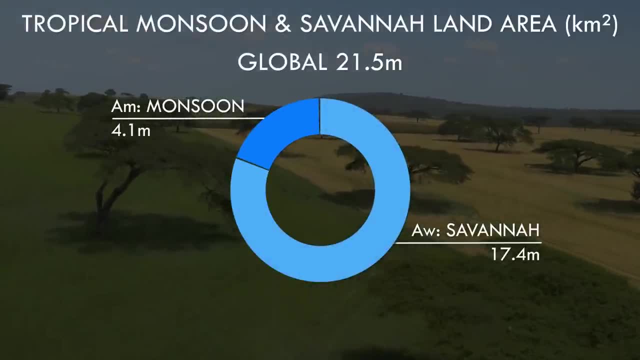 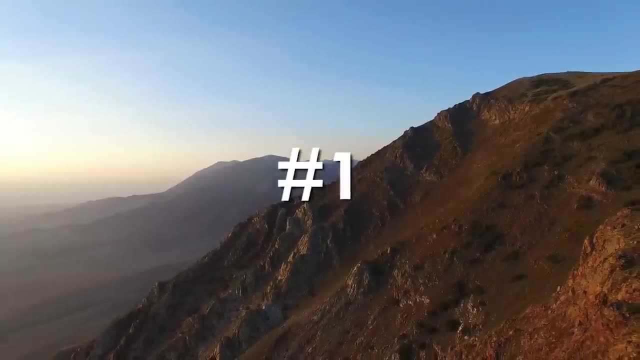 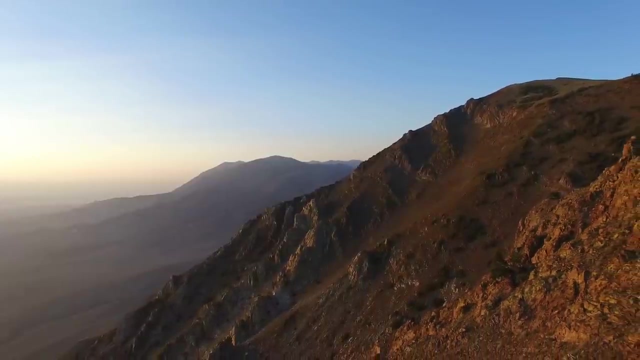 area. the remainder is just shipping, And so we come to the world's largest climate zone By a process of elimination. you might have guessed what it is, and it's a fact that might bring you some concern, with all the talk of climate change. 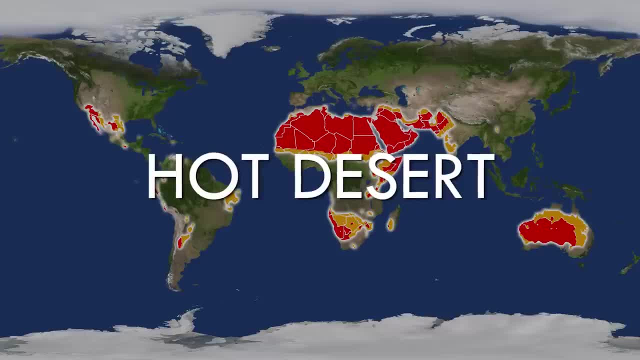 Because the most extensive climate regions on Earth are the hot deserts, making up a full fifth of all continents. But if we look at the continental land areas- the Sahara itself being half of that- the scorching arid lands of the subtropical regions of our planet can appear deceptively smaller. 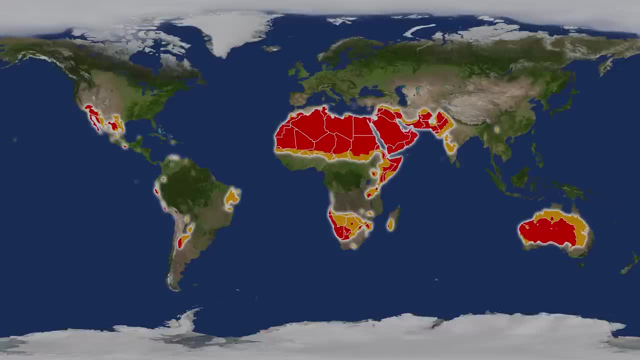 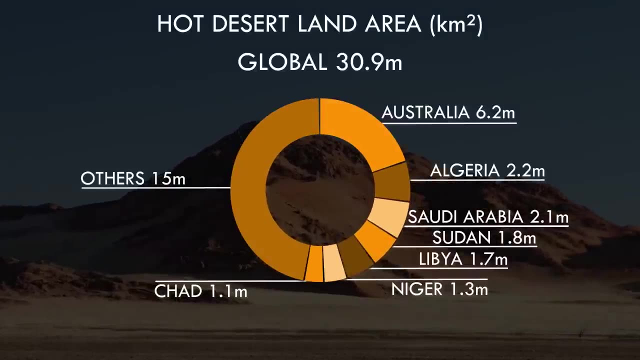 than the subarctic regions on a map because of errors in projection that cause more polar regions to appear larger. When looking at the distribution of these lands, it's not surprising to find countries adjoining the Sahara dominating, although the single largest contributor is the land. 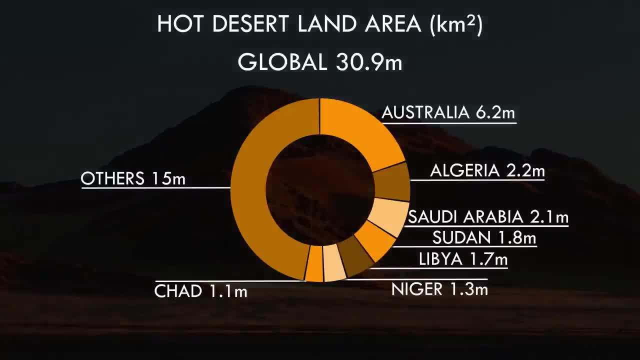 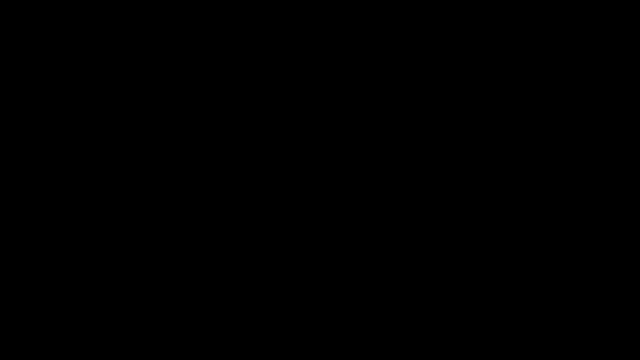 down under, whose continental bulk is made up predominantly of desert That dominates over its slightly wetter, semi-arid form, as this chart shows. So with our list complete, let's now make a comparison of our 12 grouped zones in our 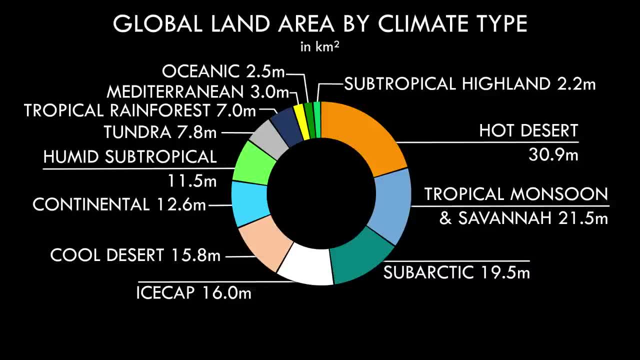 final graphic. There are two notable patterns here. The first is that almost half of the land on Earth is practically unusable by humans in the form of arid desert, ice sheets or tundra. The second is that the three smallest zones combined are barely bigger than the next largest. 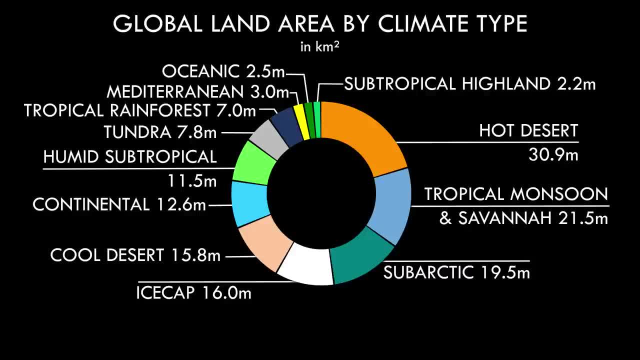 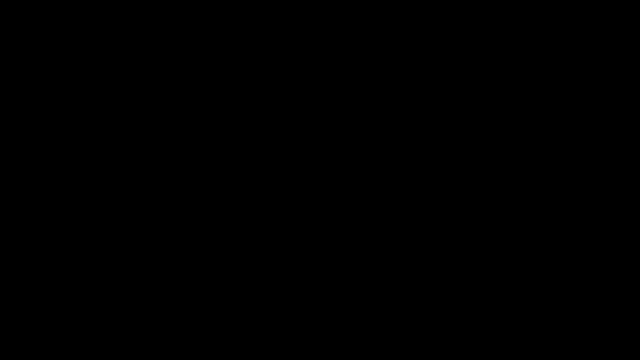 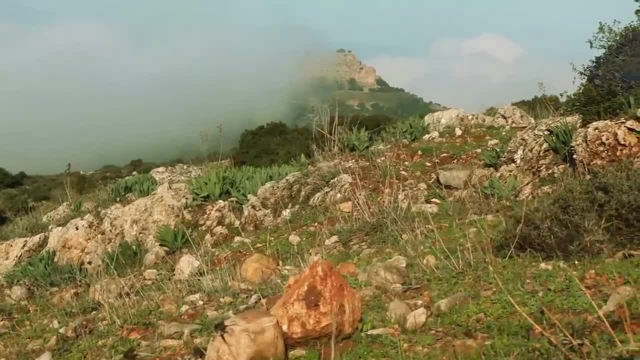 and yet these zones continue to dominate. So if you're from one of these regions, like I am, don't feel bad. Remember, small is beautiful, So I hope you enjoyed this tour of Earth. in respect to climate and land area, Once again I'd like to thank Richard Torres for compiling the data on carbon climate areas. 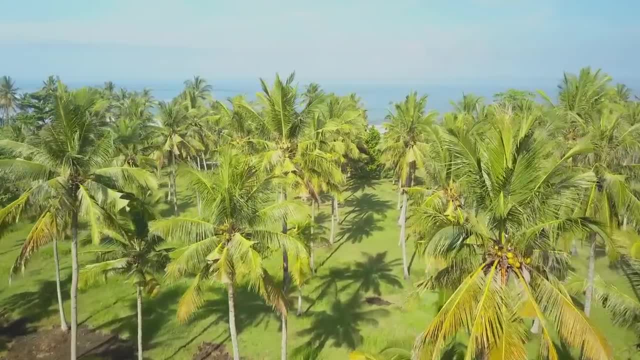 by country. Please like and share this video if you found it useful, and don't forget to subscribe to my channel so you don't miss future episodes. And if you fancy supporting this channel, please check out my Patreon page, where you'll be able to support my work.